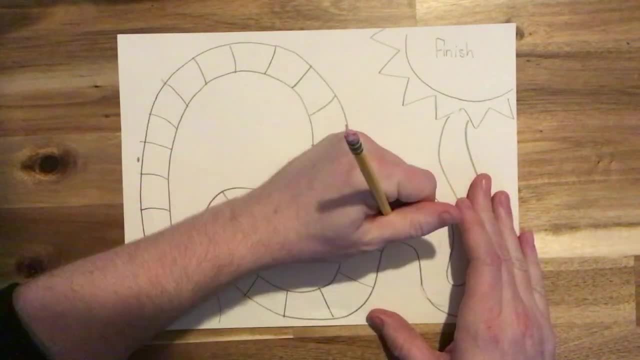 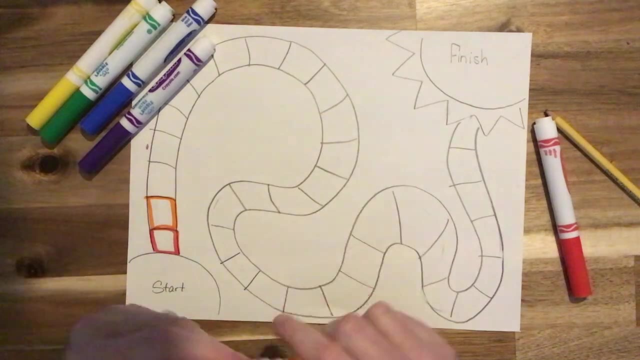 so I have different spaces for my players to land on in my game. After I've sketched it all out in pencil, the next thing I'm going to do is add color. In this case, I'm just going to add color simply by outlining each of the lines. So I'm going to add color to each of the lines and I'm 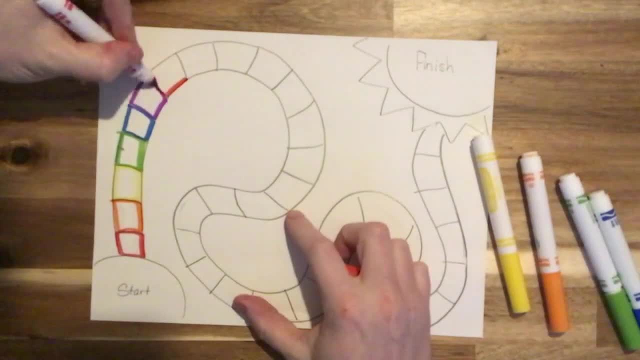 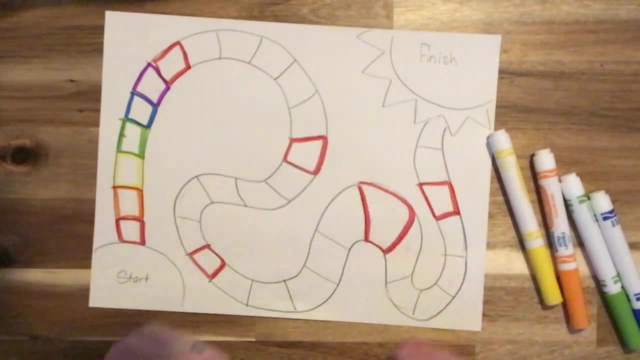 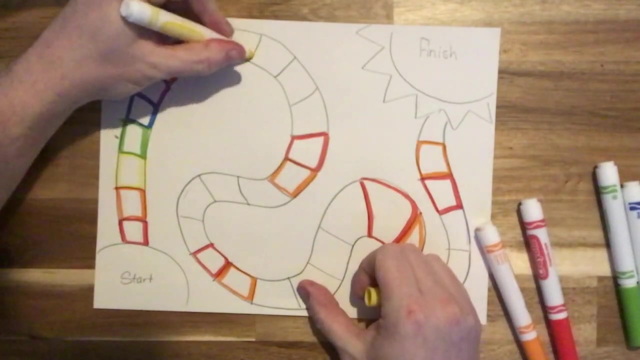 going to go in rainbow order. I'm going to use just six colors, because I'm going to create a six-sided die with different colors later on. So I'm going to just continue in that rainbow pattern of red, orange, yellow, green, blue and purple until I've covered all of my spaces on the board. 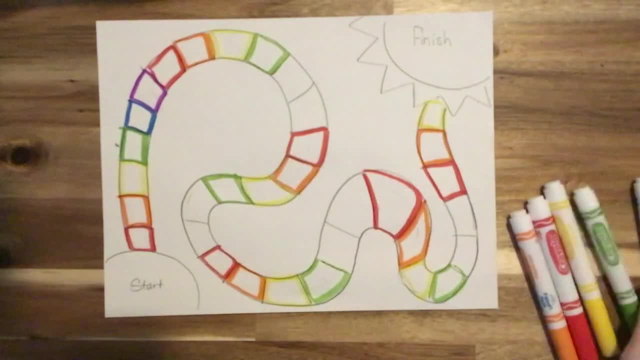 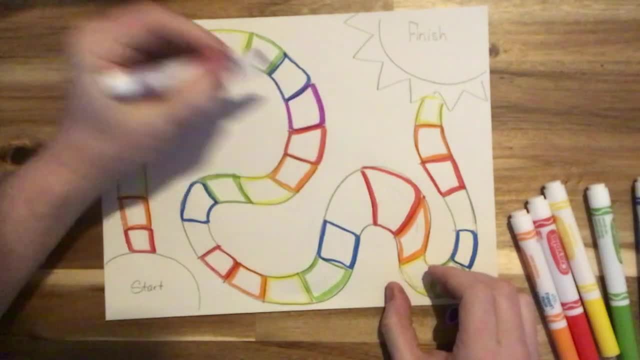 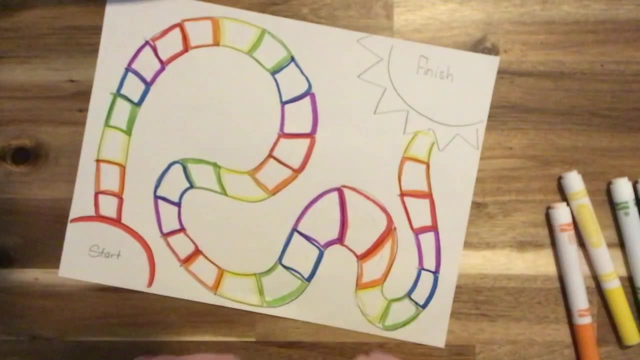 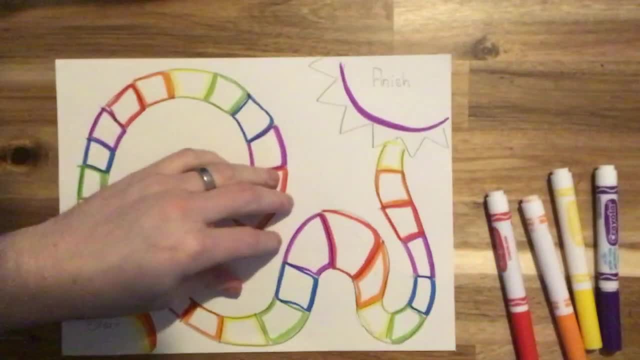 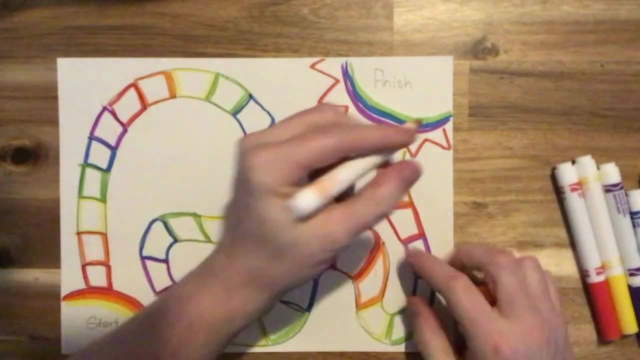 Candyland. you might land on a certain spot and there's a shortcut up to another place, or chutes and ladders you move forward and back across the game board. So I might create some spots that are teleportation stations and maybe they're. 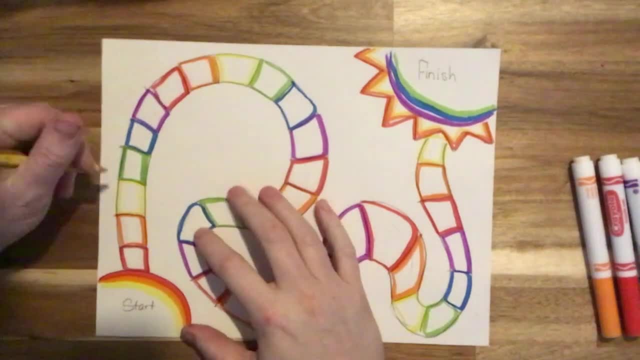 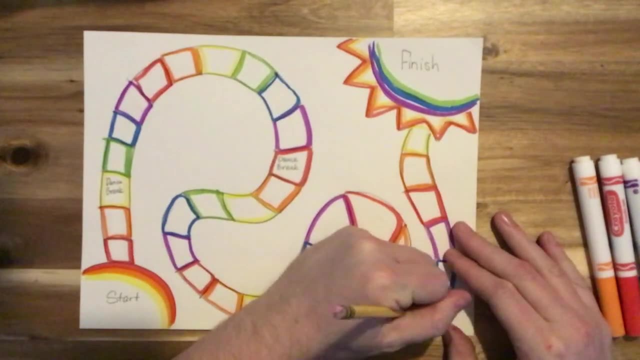 If I land on a certain spot, there will be a dotted path to another spot, Or I might decide that I'm going to have a dance break spot on my game board. So when I land on that spot, everyone has to take a break and just dance for a minute. 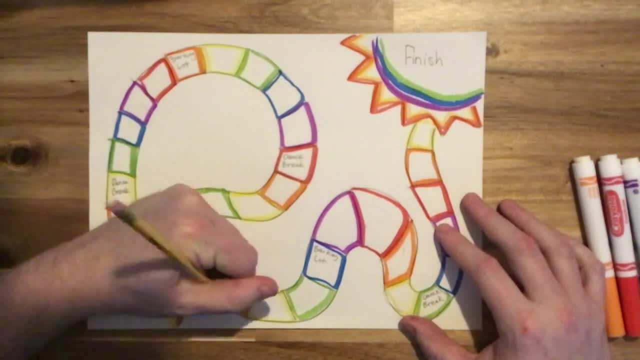 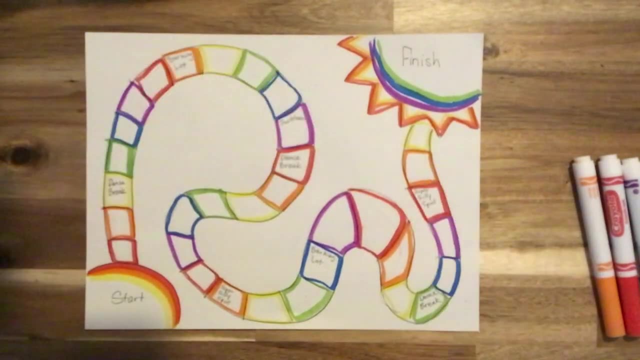 Or I might create a super silly spot and whenever you land on that spot, you just have to do the silliest thing you can think of. I would encourage you to think outside the box and just think about what would be something fun. that breaks up the game. 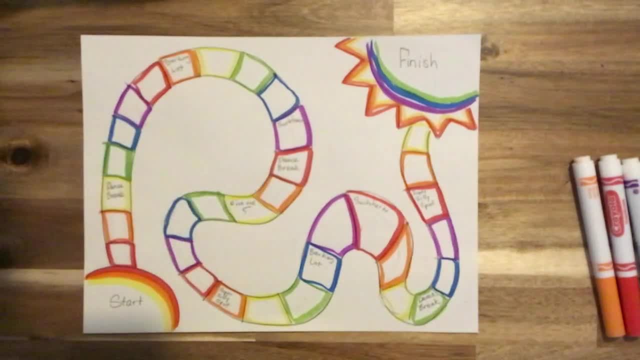 Maybe you're going to have a spot that's your barking lot and anyone who lands on that has to bark like a dog until their next turn. It's up to you, but think about things that will make your game have an unexpected twist, because that can make it lots more fun. 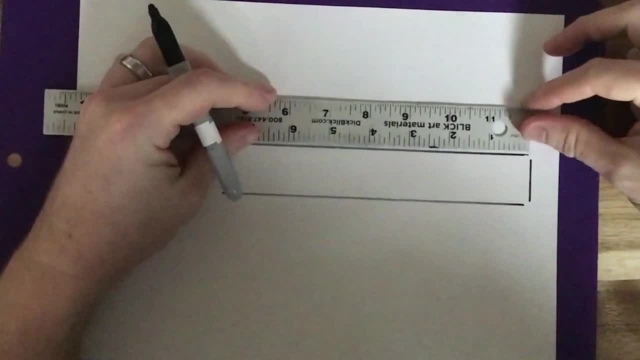 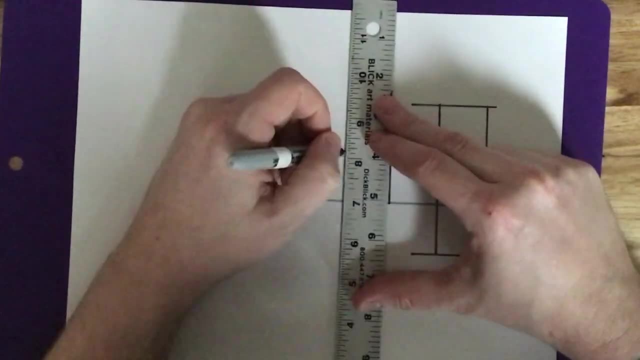 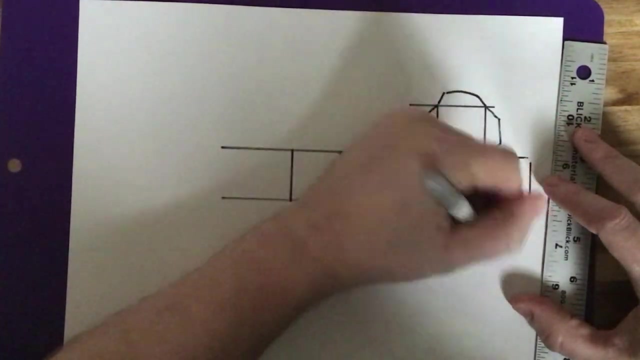 Now that I've designed my game board, I need to design my die, So I'm going to use my ruler and, for simplicity, I'm just going to use the width of the ruler as my units And I'm going to make basically like a lowercase t that is five units wide and three units tall here. 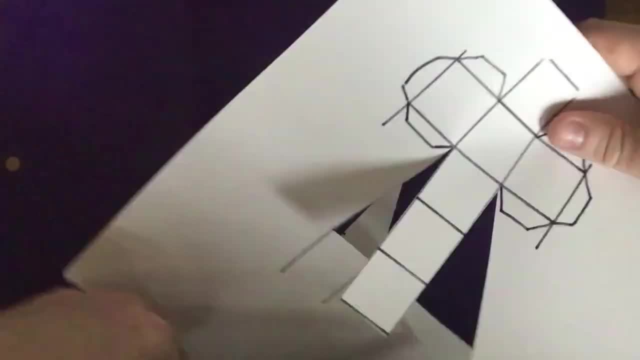 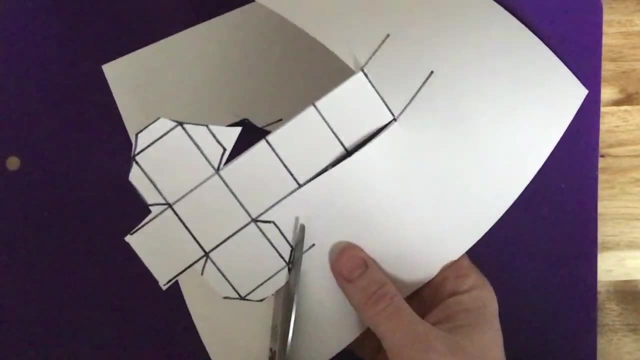 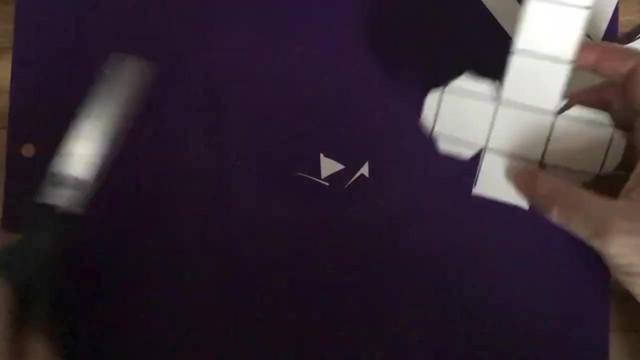 And then I'm going to cut it out. I want to leave a little bit of extra for my glue tabs around those two spots, Those two spaces that are going off to the sides, and I'll get to that a little bit later. After I've cut out around the perimeter, the next thing I'm going to do is color the sides of my dice. 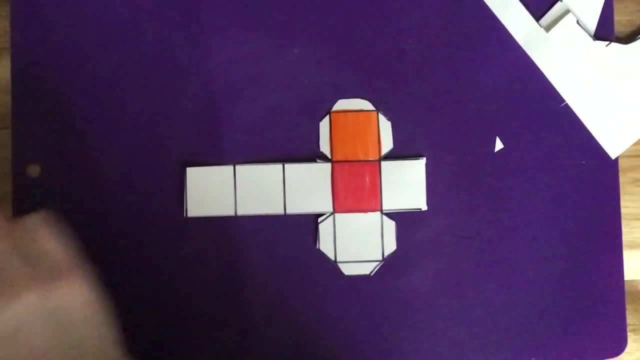 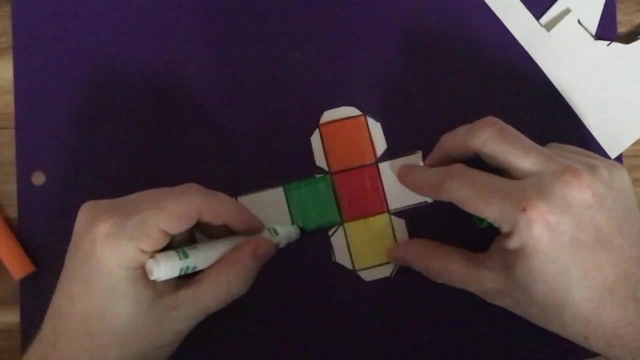 I'm going to make one red, one orange, one yellow, one green, one blue and one purple. That way when I roll my dice it will tell me where my player should land, Go to the next red spot or the next blue spot or the next purple spot, etc. 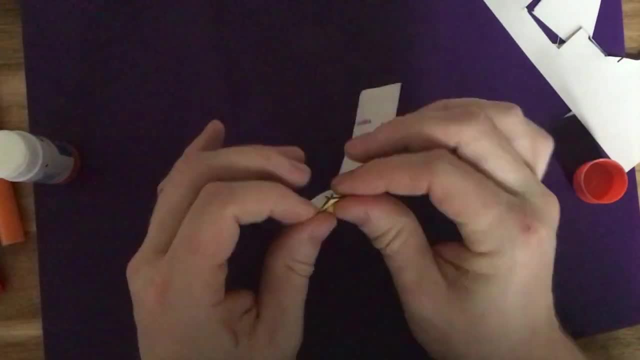 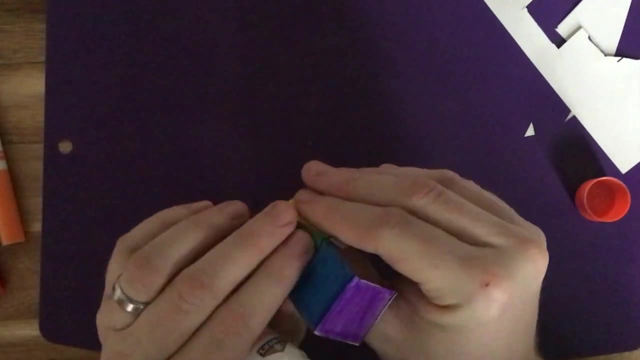 It's basically like the candieland system, except I don't really want to have to deal with all those cards, So a die seems like a simpler mechanism. The next thing I'm going to do is crease on all of those lines. 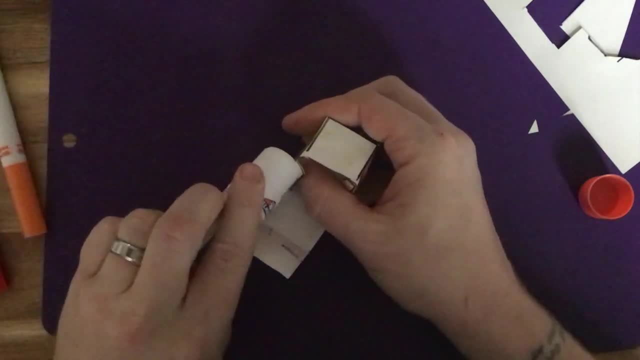 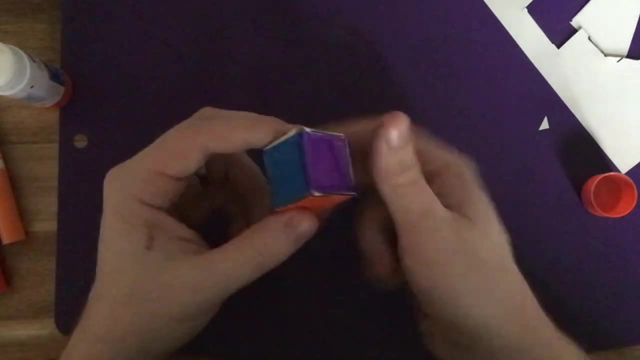 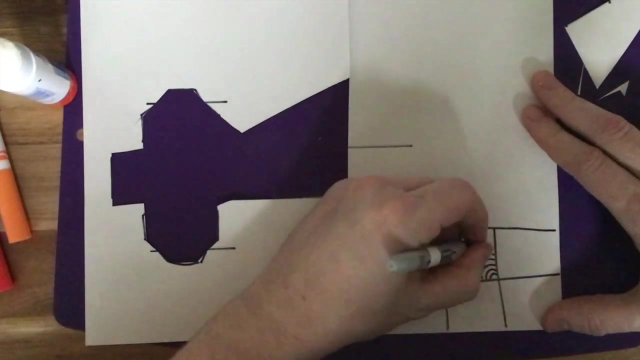 And I'm going to put glue on those glue tabs to glue the sides together to make a cube. After I have my colored cube for our dice, I'm going to make my game pieces. ي I'm just going to make four game pieces and since I have so much color on my game board, 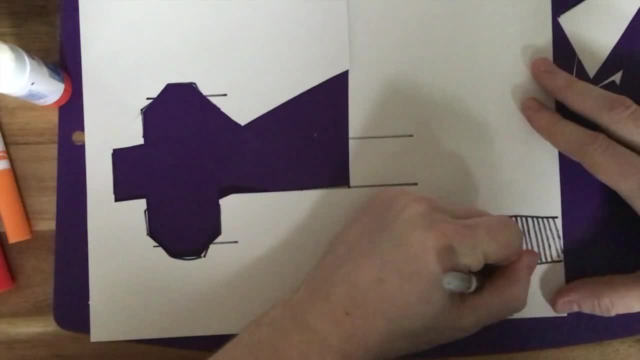 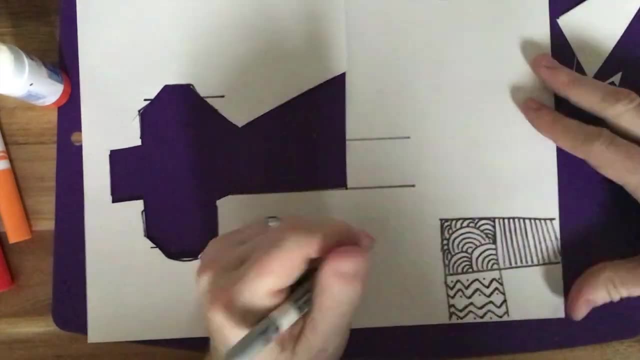 I thought it would stand out more if I make my game pieces black and white. I'm just making four squares that have different patterns, different kinds of lines and dots on each of those. So I got to get a little bit creative, thinking about what kinds of different patterns can. 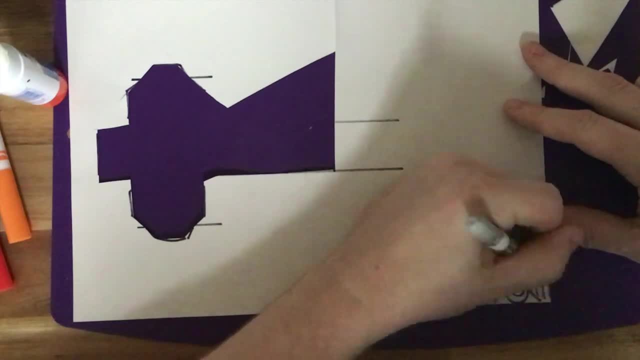 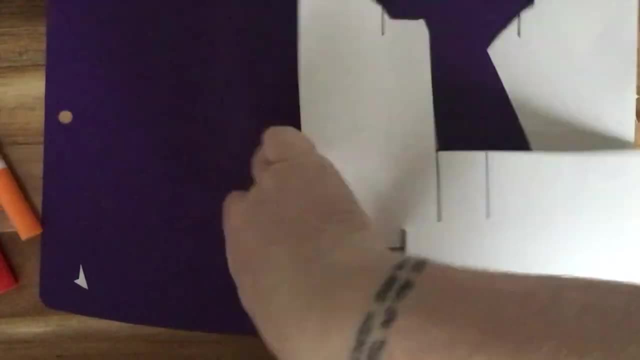 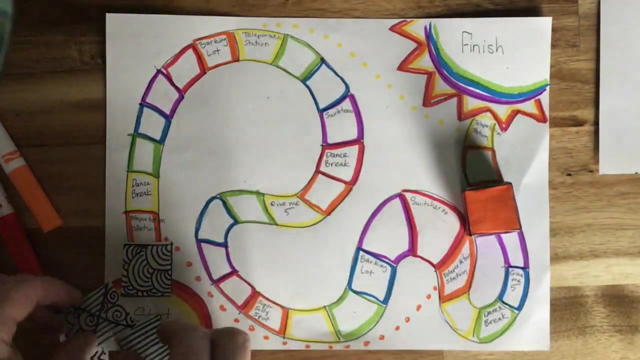 I make to make each of those game pieces look different and unique so each player knows which piece is theirs After I've designed them, I'm obviously going to cut them out. Now I have all the pieces that I need to play my game. think about what gaming elements. 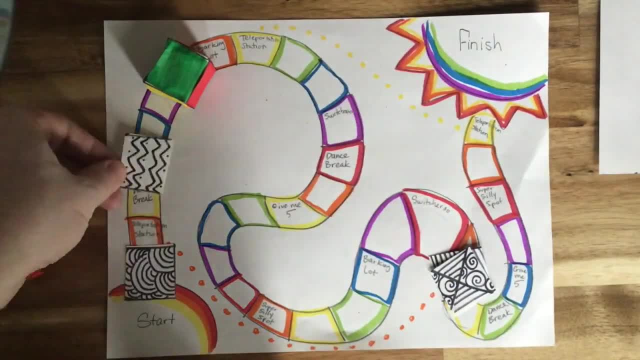 you like and how you can combine them to create your own new and unique game.